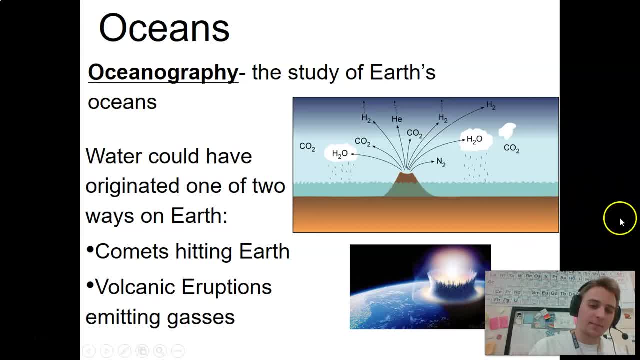 This is one of two ways it could have come: Either comets hitting the Earth or volcanic eruptions emitting gases into the atmosphere. Probably both, actually Probably both. So either comets coming hitting Earth and bringing water with them and water going up to the atmosphere, or water that was trapped in Earth's surface- Excuse me- underneath Earth's surface that came up during volcanic eruptions and converted into H2O. 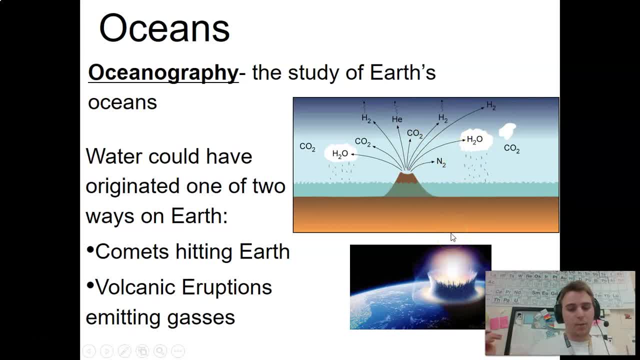 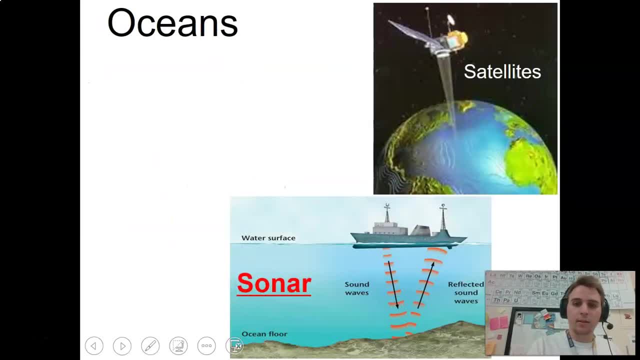 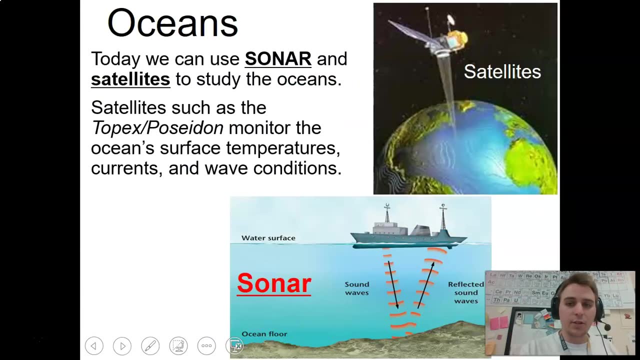 into vapor, which then rained down And you wouldn't think about it. but raining over billions of years, that's going to create some oceans. Okay, So, All right. So today we can use sonar, sonar, sonar and satellites to study the ocean. Satellites such as Topex, slash, Poseidon, monitor the ocean surface, the temperatures, the currents, wave conditions, sonar and 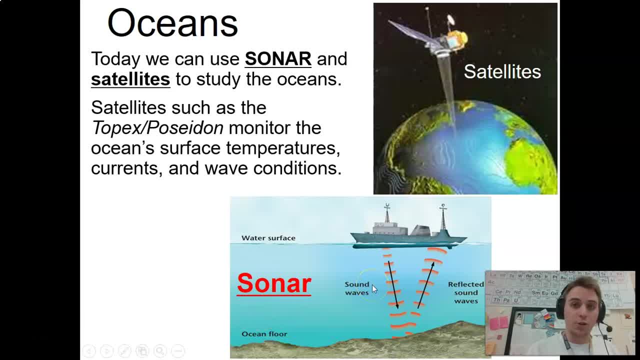 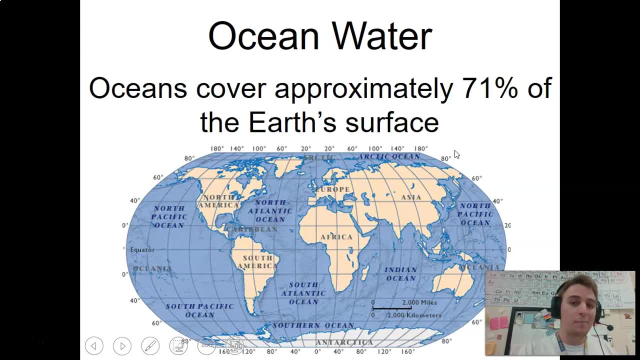 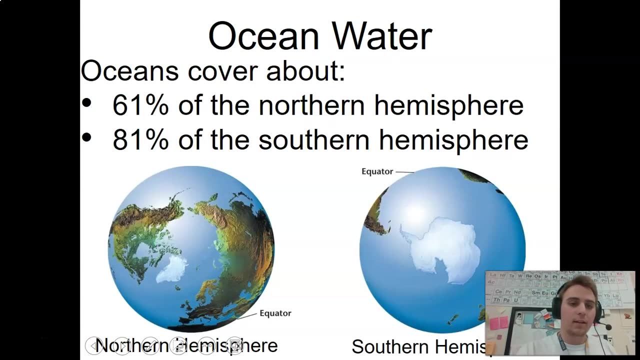 as you can see down here, allows us to map the ocean floor. Okay, As I said, oceans cover approximately 71% of the Earth's surface and make up right around 98% of all of Earth's water. Okay, See this for the hemispheres- 61% of the northern hemisphere, 81% of the southern hemisphere- If Antarctica wasn't there, which a lot of people forget that it is. 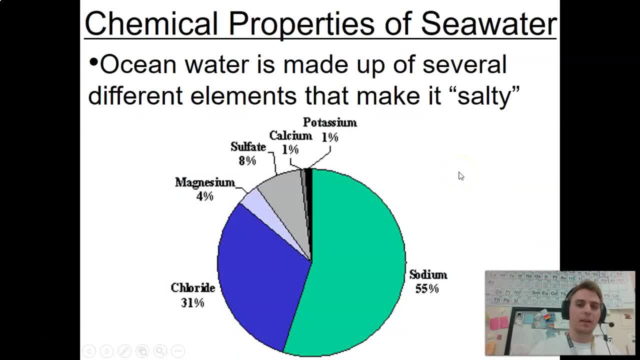 Okay, All we would pretty much have down here is ocean. Okay, So what makes seawater salty? It's a question I get a lot whenever we go over ocean stuff. So ocean water is made up of several different elements. Okay, Primarily it is water, but what is dissolved in there is a lot of sodium, a lot of chloride, which should make sense. Sodium chloride is salt. N-A-C-L is salt, straight up salt like you would have at your table. But there are also 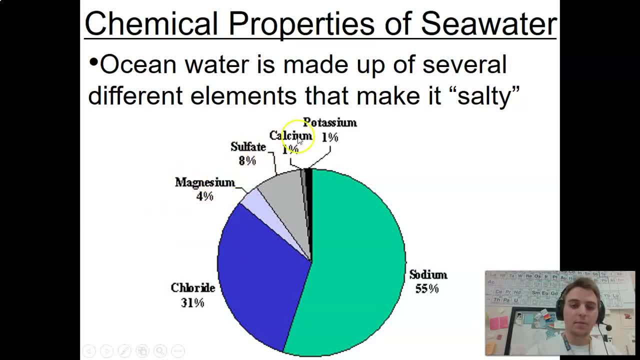 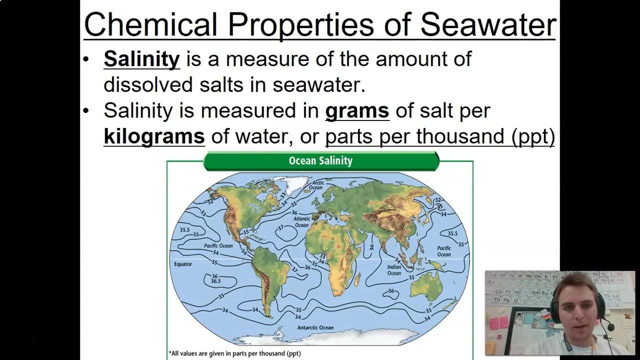 other elements like magnesium sulfate, very small amount of calcium and a small amount of potassium, As well as less than 1% of any other kind of things that might dissolve in there. Okay, Now, when we talk about seawater, we need to talk about a couple of chemical properties. Okay, 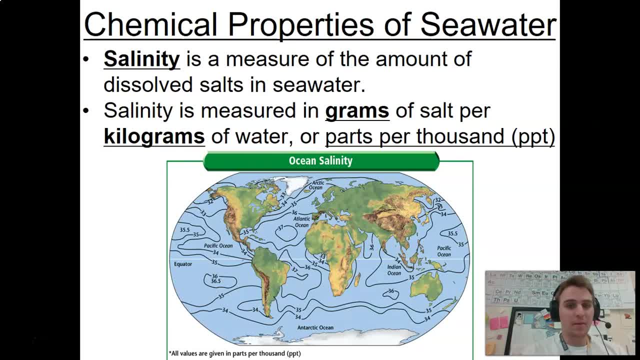 Okay, Anything. salinity is a word, it's a term that means how much dissolved salt is in the water, And salinity bone count is 25.ает. grams or kilograms? okay, usually it's grams of salt per kilogram of water or parts per thousand. 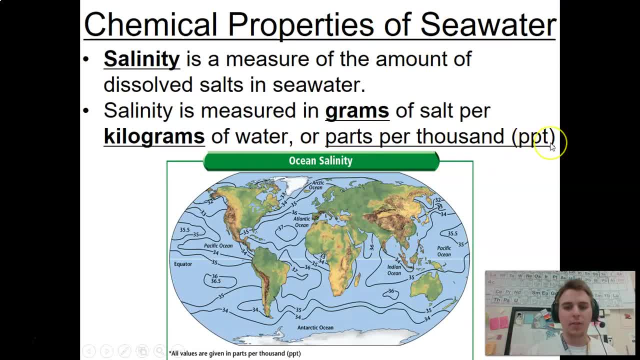 ppt. okay, so remember that. parts per thousand, all right, and if we look at this, we can actually see differences in ocean salinity, uh, in different areas. so all these values are given in parts per thousand, as you can see, but on this map close to, uh, the north of here, up by alaska, it's actually 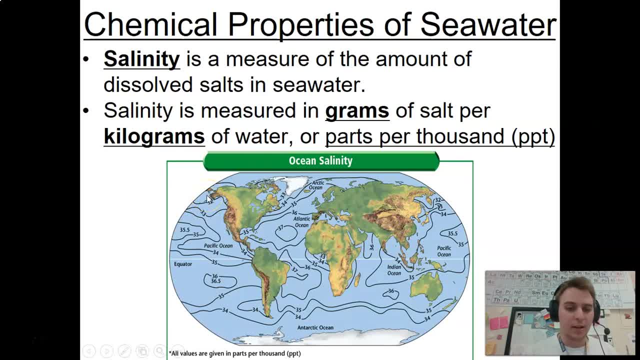 less salty, it's right around 32 parts per thousand, whereas in the saltiest places it's going to be right here, off the coast of south america, of brazil, or right here, right in the middle of the atlantic ocean between north america and africa- it's at 37, so you're not seeing a huge difference. 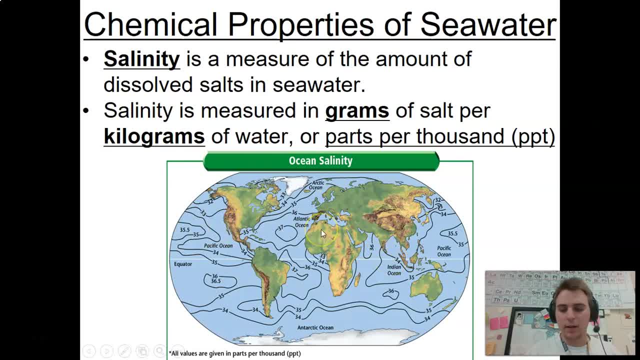 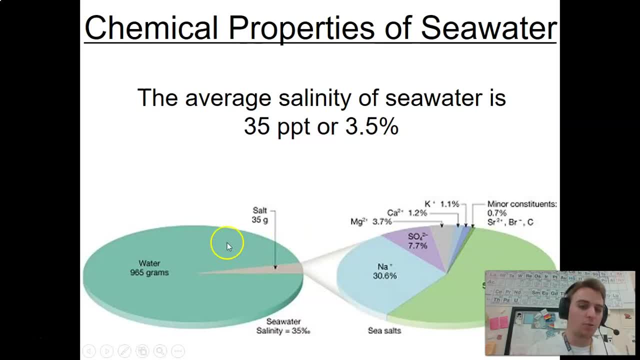 uh, anywhere in the oceans. but there's a difference. average salinity of seawater is right around 35 ppt or 3.5 per cent. so mostly water, but still about 35 or, excuse me, 3.5 percent of the salts. and again this is. 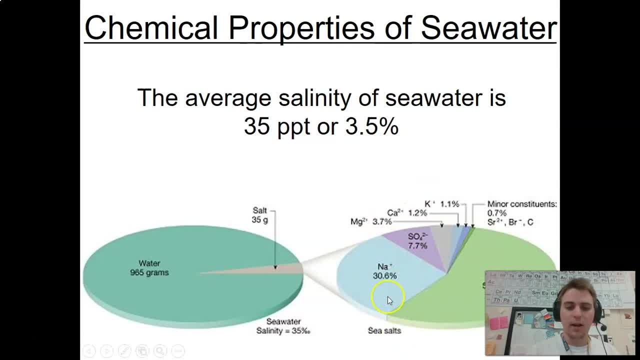 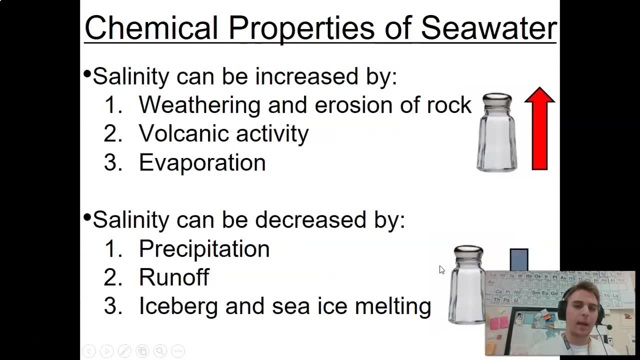 lots of different things. it's not just sodium and chloride, it is also sulfates, calcium, magnesium, like i said, all those other things okay. so how do you add salt in? how does some water get more salty, how does some get less? so salinity can be increased by weathering or erosion of. 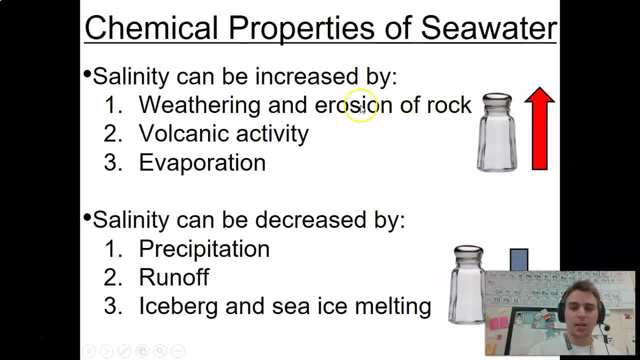 rock. okay, which should make sense, because the salts can come off of the rock and go into the ocean itself. volcanic activity that's going to be adding it directly into the ocean. water from the minerals that are being erupted, and then evaporation, so, as the water goes away, what's left behind is the salt. 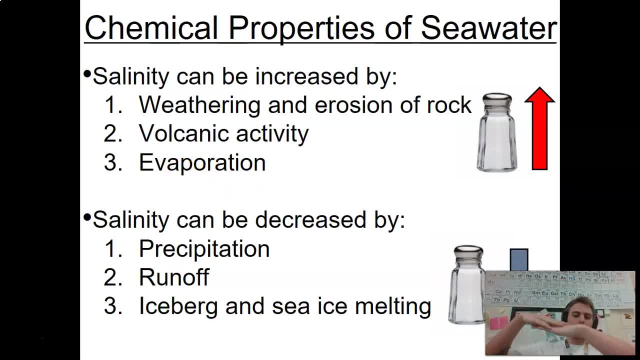 okay, so normal evaporation. you've got, you know, the water right here, and as the water goes away, all the salts are left behind. salinity goes down by precipitation, so adding fresh water back in runoff from fresh water sources. so rivers leading into the ocean and then icebergs and sea ice melting. so anywhere near Antarctica or in the 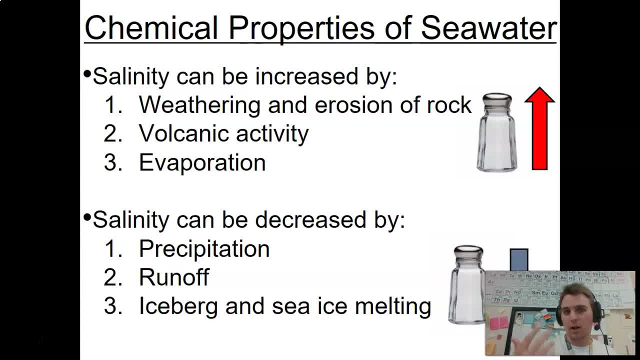 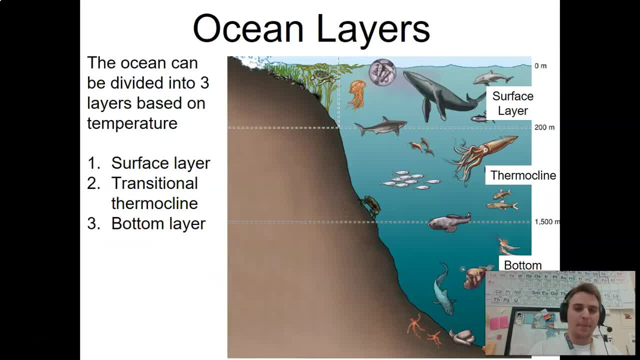 polar ice caps as that melts that. all that is fresh water. so that would decrease salinity, make it less salty. so that would decrease salinity, make it less salty. Okay, So the ocean can be divided into a number of layers. Okay, So three basic layers based on temperatures. This is actually how we divide our ocean, Usually based on temperature. A lot of people think it's based on light And there are divisions based on light, But it's on temperature is what we're going to be worrying about for this video. 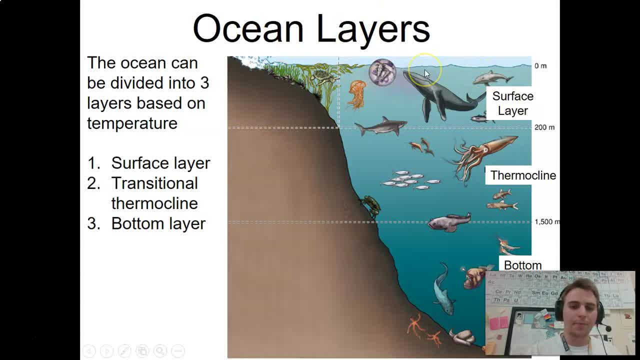 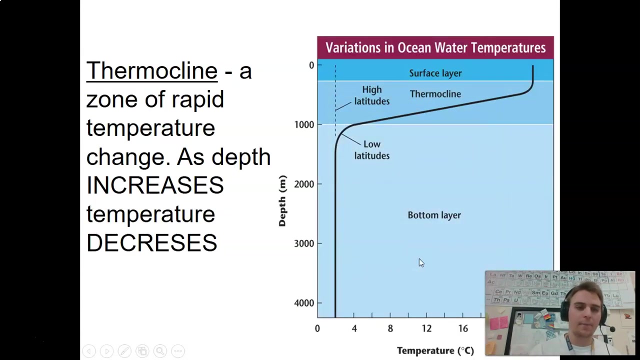 So the surface layers right up here, Nice and warm, Okay, This area is called a transitional thermocline. Okay, Therm means heat or temperature. Cline is usually going to mean a change over some distance, So that it's a decline or an incline. So this is a thermocline: A change in temperature in the bottom layer down here. Okay, Yeah, Here you go. 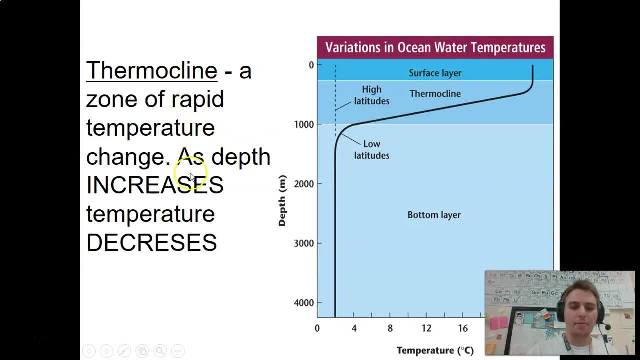 Thermocline is a zone of rapid temperature change. So as depth Increases, Temperature decreases, And that is because of the lack of light that is able to penetrate that deep. The light Filters in just so far and after a little while. 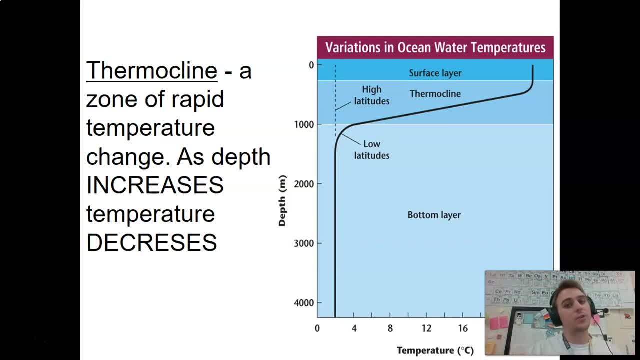 It can't diffuse anymore, So no light gets down there. If there's no light down there, It can't transfer into heat. Okay, So it gets quite cold. So the surface layer is relatively warm, See So temperature in degrees Celsius. So surface layers in some areas. 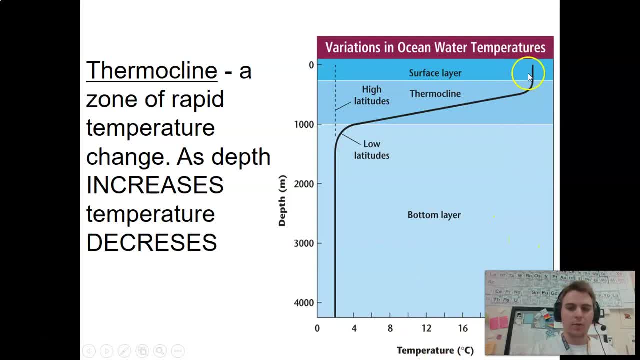 Okay, We see, is up to 24 degrees Celsius. That's pretty, It's pretty warm, That is pretty warm, That's You know, that's close ish to room temperature, I'm pretty sure. And then you've got a very rapid thermocline. 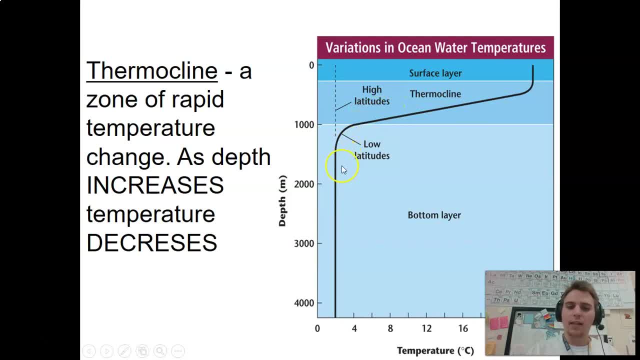 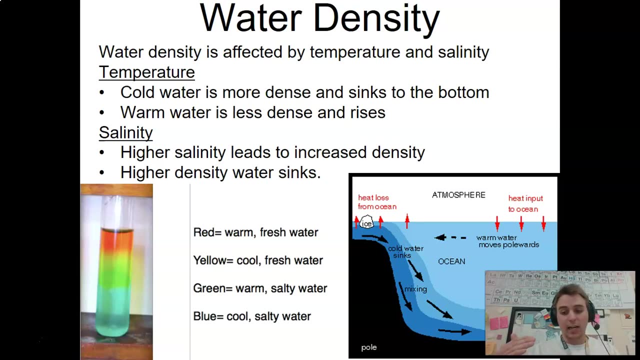 And then You've got this bottom layer and you're going to see really, really cold temperatures, much closer to almost freezing. Okay, Zero degrees Celsius, So going along with this, Okay, So going along with this, Okay, Along with temperature and salinity. 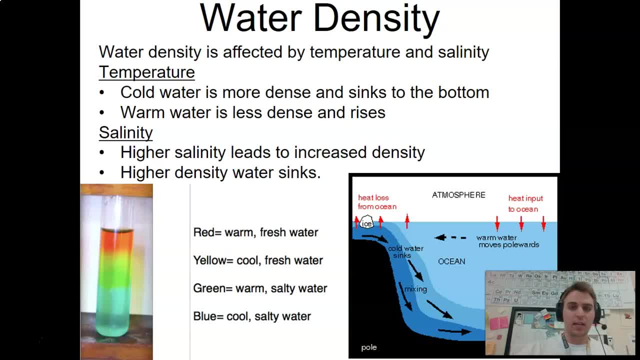 Okay, How hot, cold, salty the water is, You're going to see different densities. Okay, Water density is very affected by temperature and salinity. So cold water is more dense, And so it sinks to the bottom. Warm water is less dense. 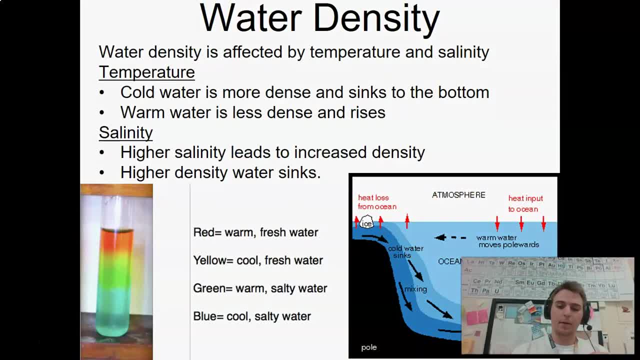 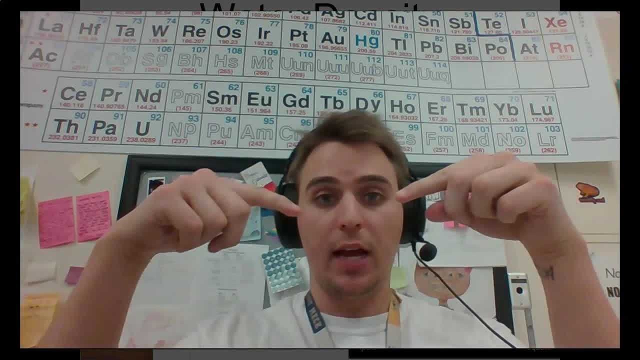 And that should make sense, Right? If you think about it, Here I'm going to make myself bigger real quick. So if you think about it, Warm water- What warm temperatures do to any fluid Is it makes it move around more. 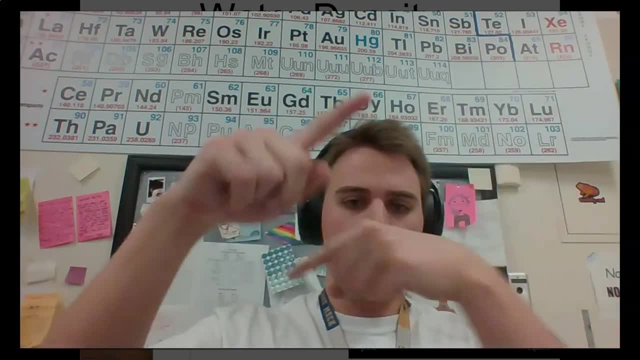 And as it does that, They're going to be Going like this Right, Moving past each other. The denser you get- Excuse me- The colder you get, The more dense it's going to be, The closer together they are. 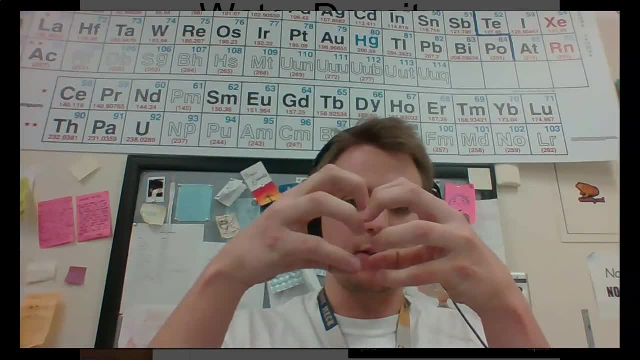 And, as we talked about before, with Magma Under the Earth's surface Density, Cause it The desert. something is, the more it sinks. Less than something is, the more Rises, And so when you put those two together, It's going to be. 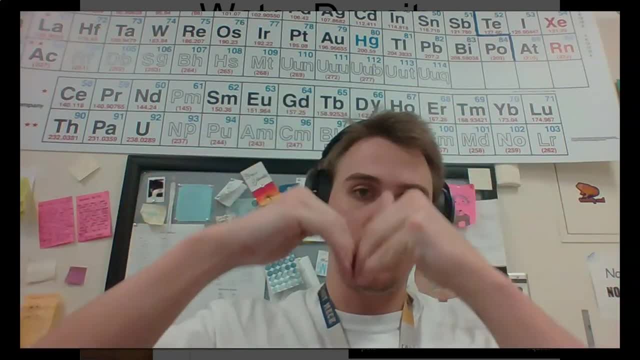 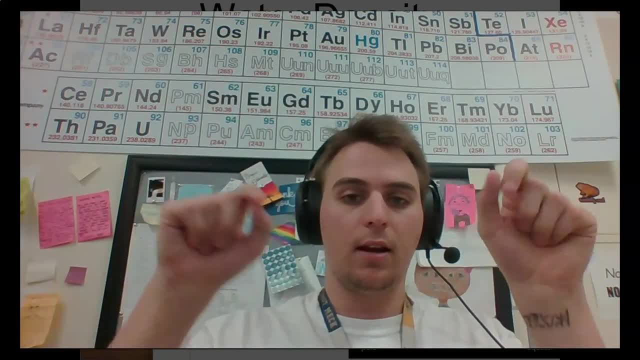 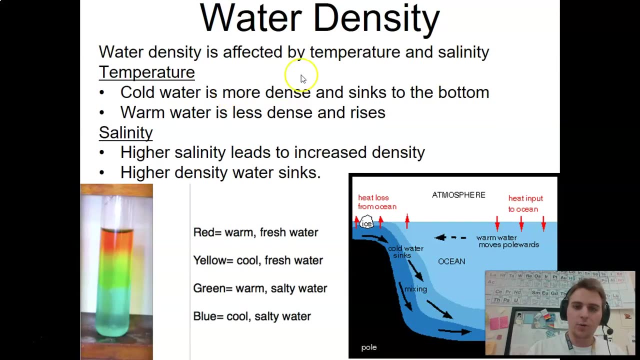 You get Convection currents, So let's go back, Okay? So warm water is less dense- It rises. Cold water is more Dense And sinks Higher Salinity. Salinity Leads to increase density. That's just because there's more stuff. 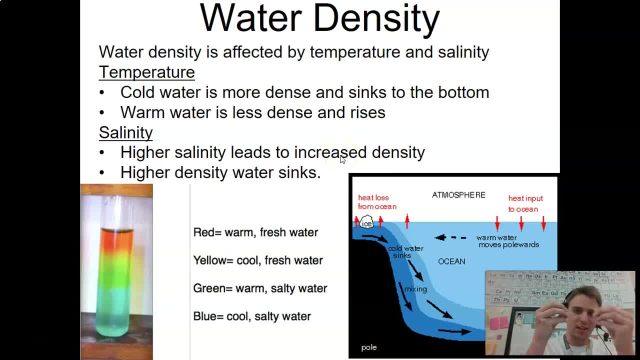 Actually In the water, Instead of it Just being water. There's other things To Which makes it more dense, Makes There Be more particles In between, And higher density water Sinks. So saltier it is, the denser it is. So if you were to put all these together, if you were to layer, 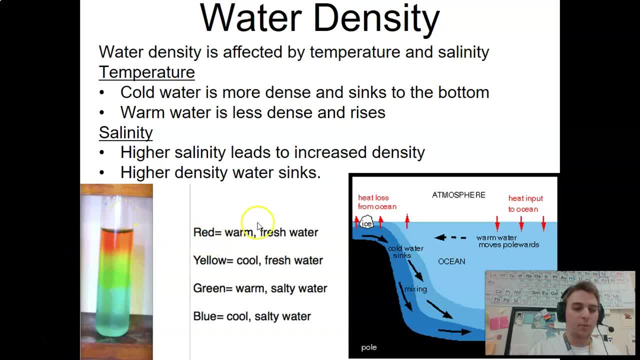 them out. this red layer would be warm, fresh water. So it is warm, making it less dense. It's fresh. no salt making it less dense. It's all the way at the top. Yellow is cool, fresh water. 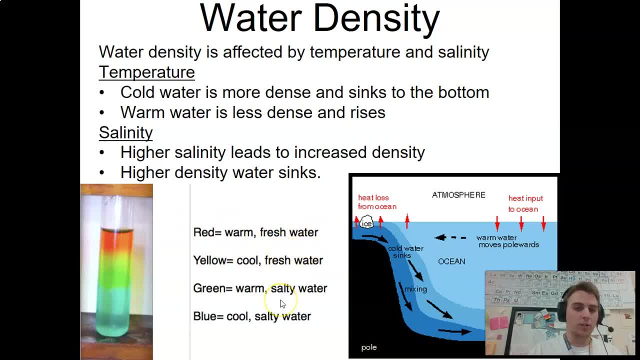 Fresh water is always going to be less dense than salty water. Always, It's always going to be less dense than salty water. Green, this layer right here would be warm salty water, because warm it's a little bit less dense than the cold. And then blue would be your cool salty water. 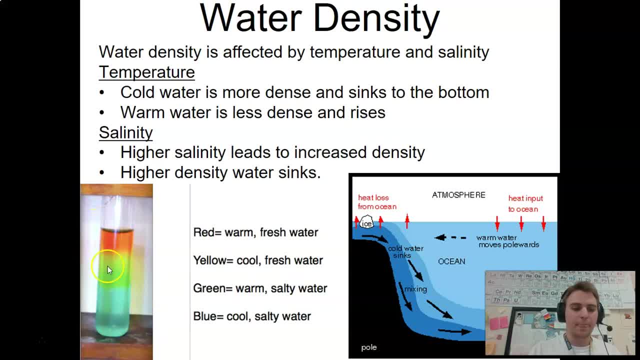 Okay, And the reason all this is important is because in this test tube it's very easy to see it like that, But on a global scale, you're going to see these different densities interacting and that's what causes the currents and the shifting waters of the world. 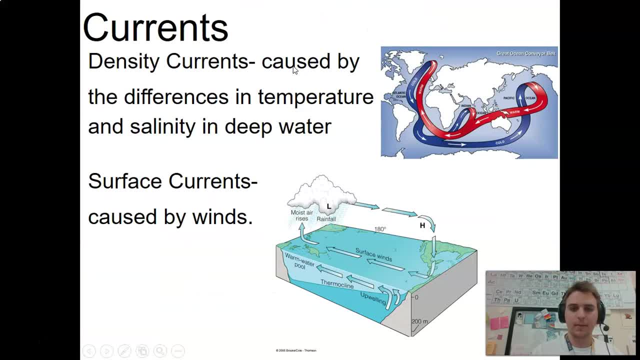 Okay, All right, Yep, So it causes the currents. So density currents are caused by the differences in temperature and salinity in the deep water. These are your ginormous, huge currents as the ocean is shifting. And then surface currents are caused primarily by wind, So wind also goes through these convection. 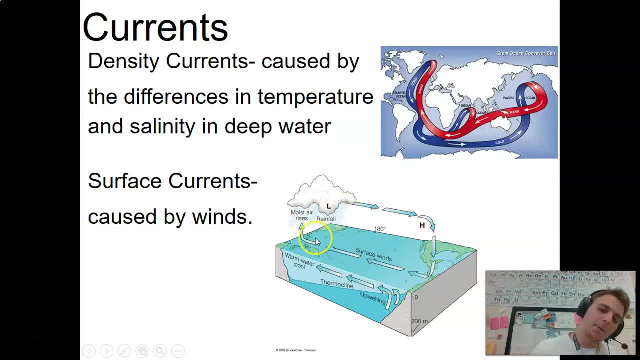 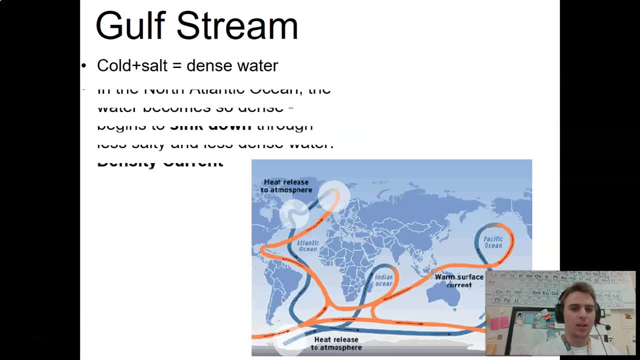 things and that can pull the water along in one direction as it does, causing a surface current. So the Gulf Stream, The Gulf Stream. This is cold and salty. Okay, It's very dense, dense water. In the North Atlantic Ocean the water becomes so. 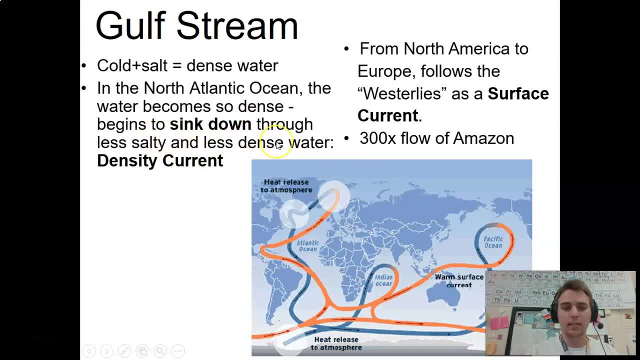 dense that it begins to sink down through the less salty and less dense water. This causes a density current. So from North America to Europe it follows the Westerlies as a surface current. Okay, So, basically, as you can see here, right in these areas, Okay, So, way down here and 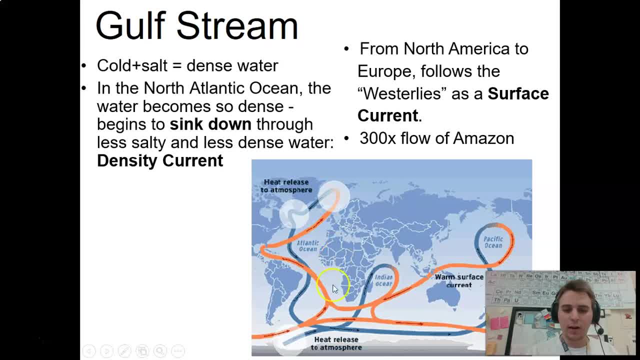 way up here is going to be quite cold. So if you follow these arrows- I know they're a little blurry, kind of hard to see- But if you follow these arrows, warm water shifting around, hitting colder areas and sinking, becoming more dense and then moving through other areas and warming up. Basically, all you really need to know there is that the Gulf Stream is an example of a density current, because cold, salty water sinks underneath the warmer water. 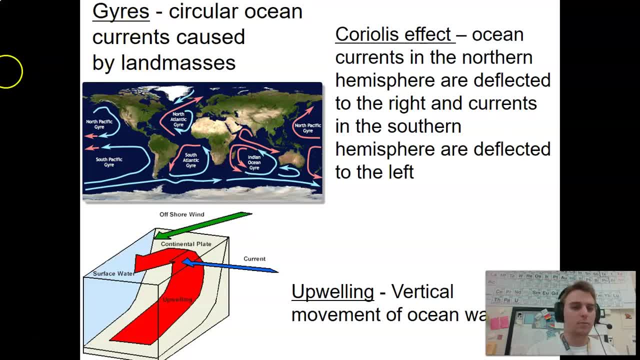 There's a couple other things we need to talk about. One is called Where's my mouse. Come back, There we go. One of them is called gyres. These are circular ocean currents caused by land masses, So this happens here in the North Atlantic and the South Atlantic, And then there's larger ones in the South Pacific, as well as in the North Pacific, and then one in the Indian Ocean. 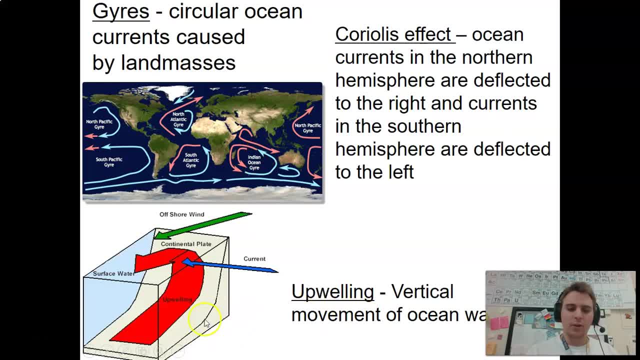 Okay, There's upwelling. This is vertical movement of ocean water. This is when it usually. when it hits a continental plate, it'll go all the way up, blast its way up like that And that'll blow up. Okay. 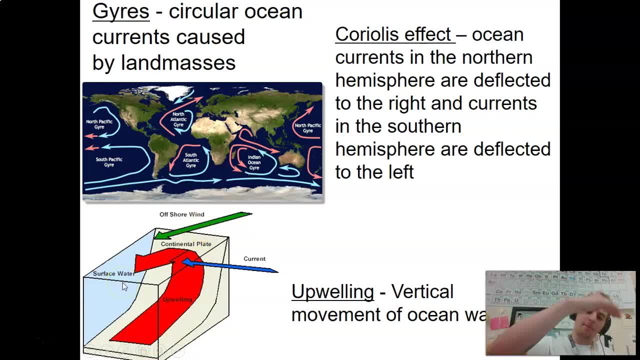 Okay, Okay, Okay, That's going to take accelerated, Okay, And it'll kick it back the other direction, causing currents as well, Or any wind that is pulling the surface water away. well, you're going to see that the ocean water is going to be pulled up to fill the space, okay, which should make sense. 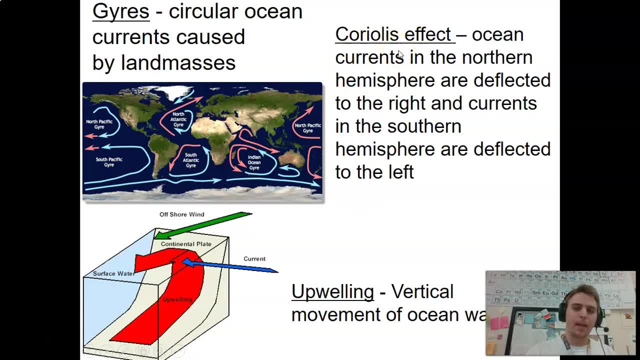 Okay, Okay, Okay. Now the Coriolis effect is — it's a really interesting idea. So this says So: this says ocean currents in the Northern Hemisphere are deflected to the right and currents in the Southern Hemisphere are deflected to the left. 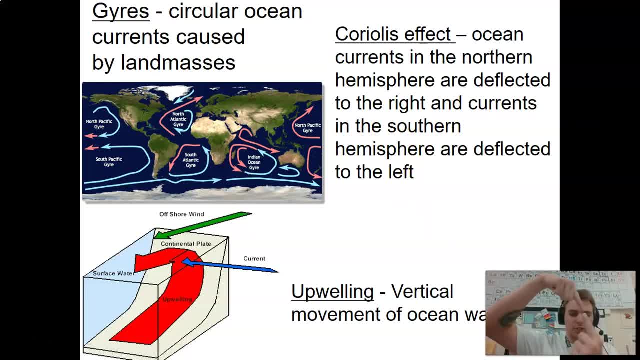 So as theilitic gas melts into the North Atlantic, it's an effect that associated to double- devolution. So as the Earth spins, okay, the Coriolis effect essentially makes it so that anything that isn't tethered down and actually attached to the Earth is going to be affected by that spin. 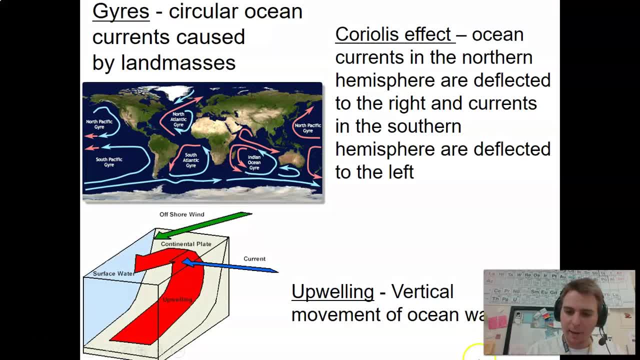 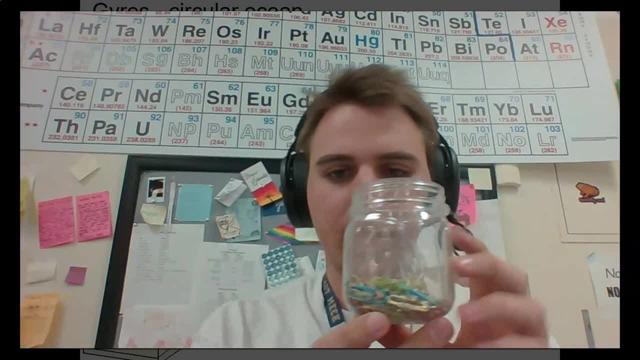 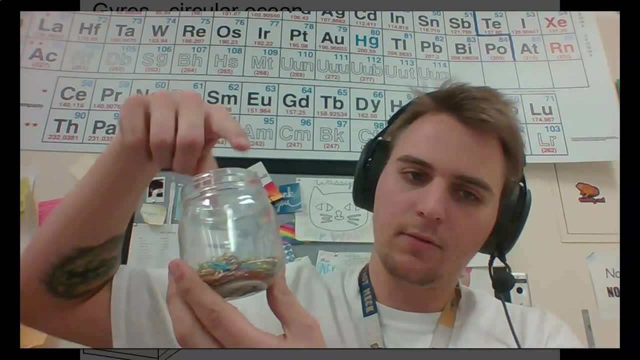 So the way to think about it- I'm going to make myself big again- The way to think about it is if this will be my example, is if this is the Earth, okay, and I decide I'm going to point in one direction. 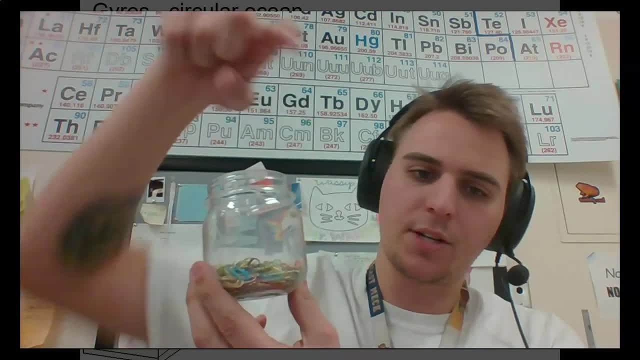 I'm not tethered to the little jar here, but I'm pointing in one direction. Well, the jar is spinning. okay, The Earth is spinning, So I'm going to make it spin in one direction. I'm going to start here. 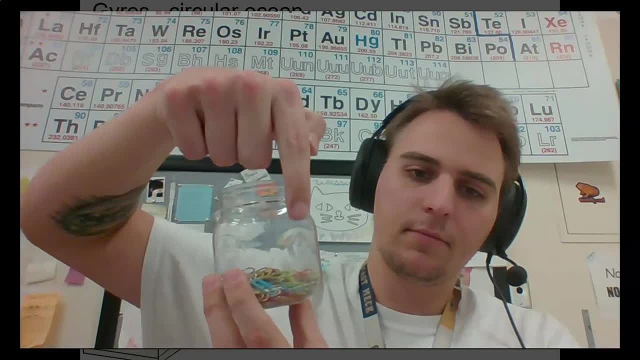 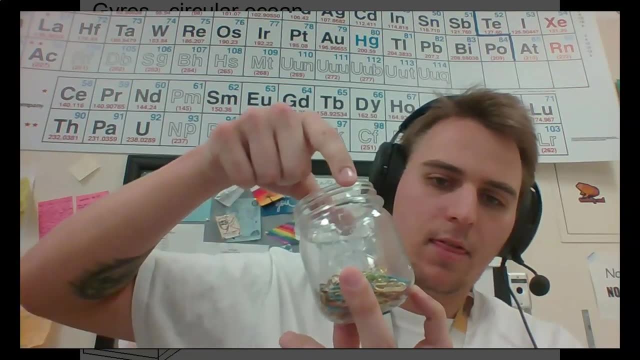 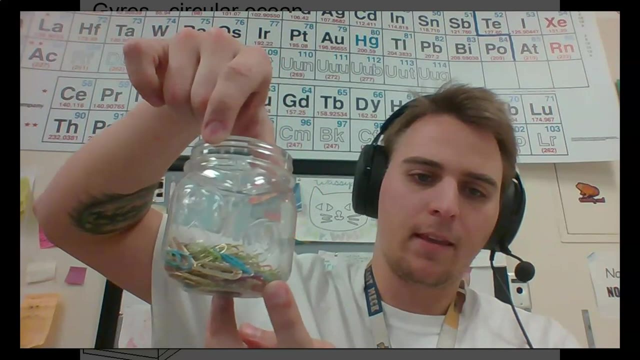 And we're going to see where I ended up. Okay, So that is where I ended up. That is where I started. I went in a straight line, but, as you can see, I ended up about a quarter of the way around the jar. 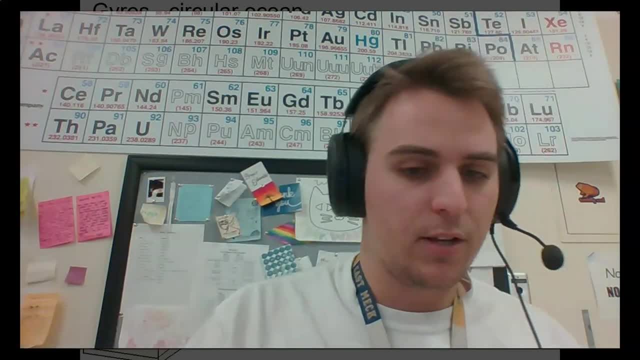 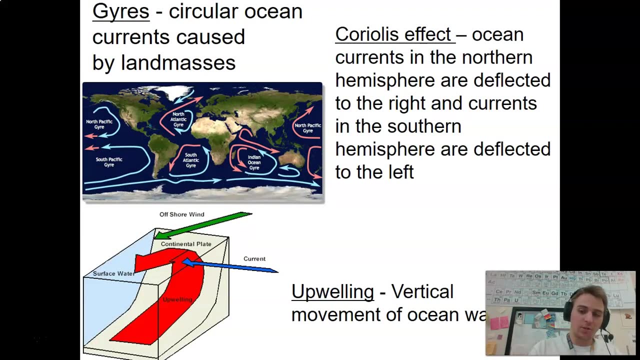 Because the jar was spinning. that is the Coriolis effect. So water in the ocean is not exactly attached to the surface of the of the world, So it is also going to be subject to the Coriolis effect where it is going to be kicked off one direction or the other because of the Earth's spin. 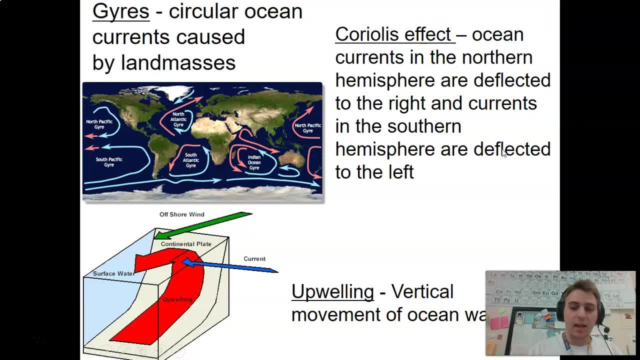 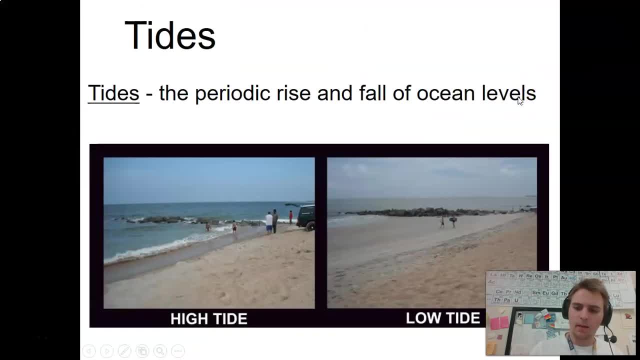 Now, if you aren't fully comfortable with the Coriolis effect, I suggest looking it up and getting a little bit more comfy. Okay, All right, We've got tides. Tides is the rise and fall of ocean levels. This is primarily caused by the moon. 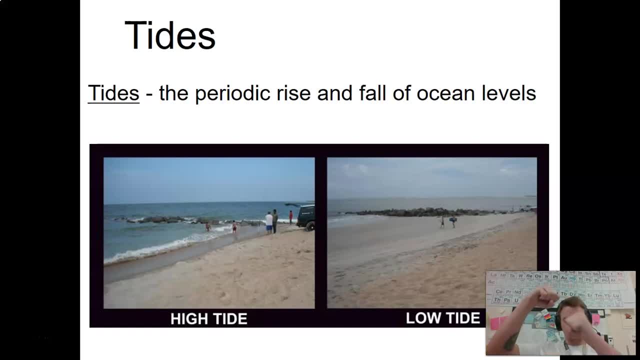 Okay, As the Earth is spinning, the moon is going around it kind of like this, And, as that happens, it's going to be pulling on the ocean as well as having the sun have its own gravity pulling on the ocean as well. 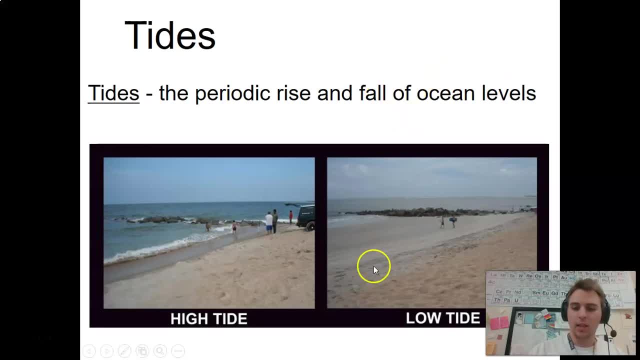 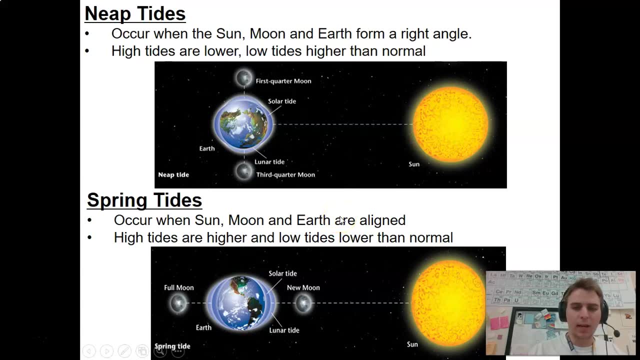 So it's going to cause a high tide at certain times of the day and low tide at other times. Now I've got neap tides and spring tides. I don't really want you to worry about this too much, because we're going to hit it again in astronomy.